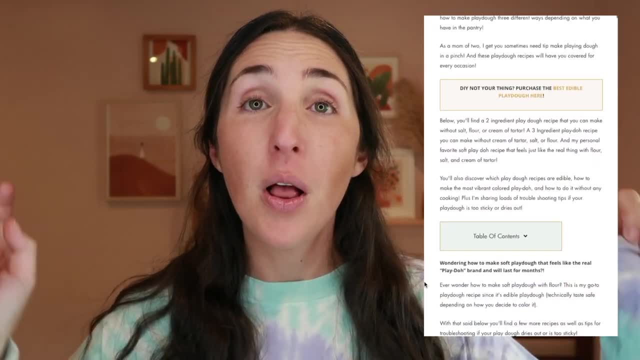 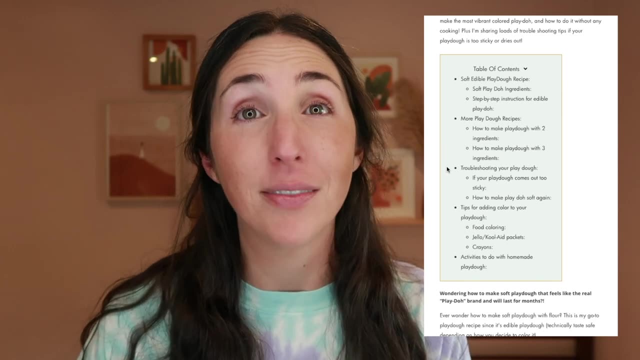 also have a blog post, so if you need to go back and reference anything in this video, that will be linked in the description box below. And it also has two more playdough recipes in case you don't have some of these ingredients on hand, And at the end of this I will also talk about 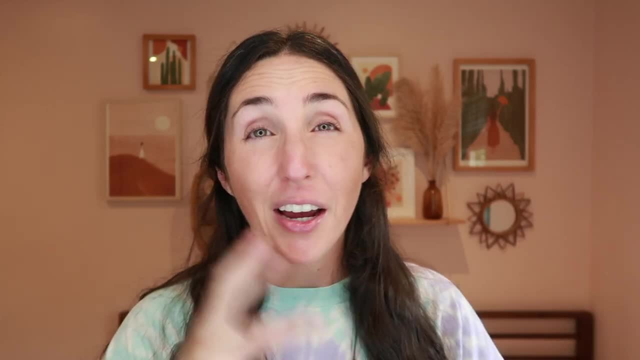 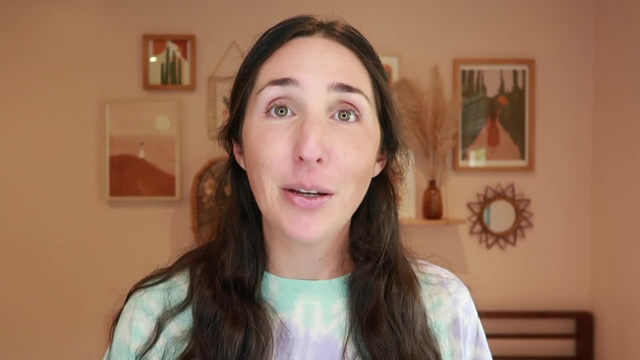 ways to troubleshoot your playdough recipe. so if it comes out too dry or too sticky, we're gonna get there, Plus tips for creating the most vibrant colored playdough. If you guys don't have time to make your own playdough, I will recommend the brand The Dough Project. 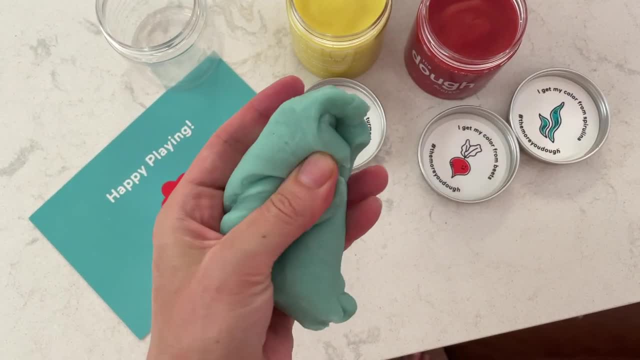 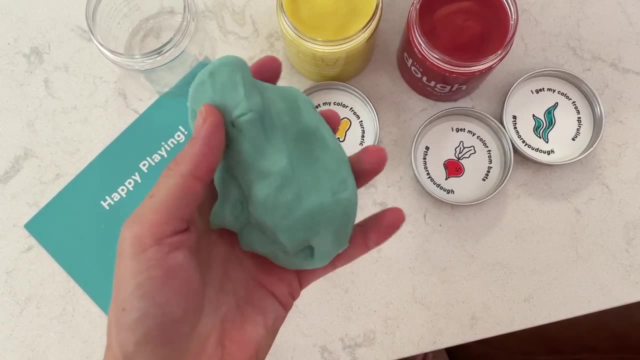 and I will leave a link in the description box below. They use food to color their playdough. so think beets, turmeric, spirulina, all that good stuff. So if you are looking for a store-bought edible playdough, you can go to The Confused Millennial. I will leave a link in the description. 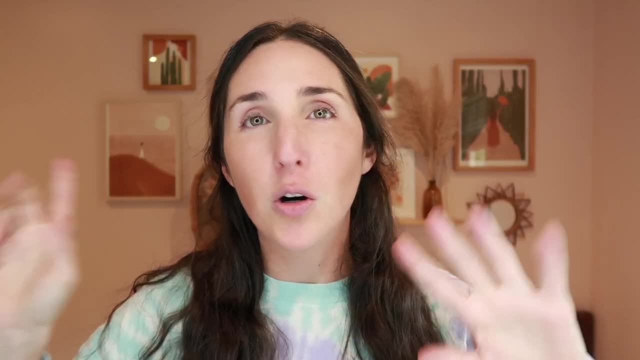 box below. That is my go-to branch and I like to have a few jars at home just in case I don't have time to make playdough. All right, let's get into it. For this playdough recipe you are going. 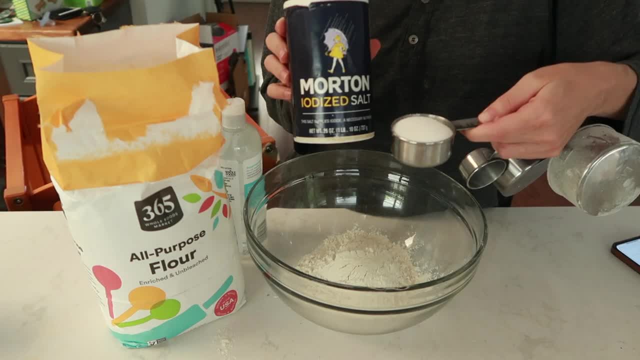 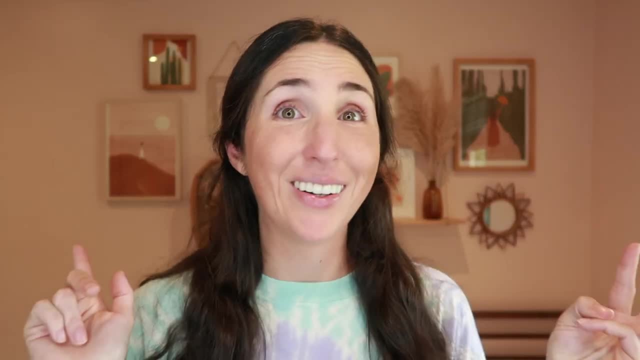 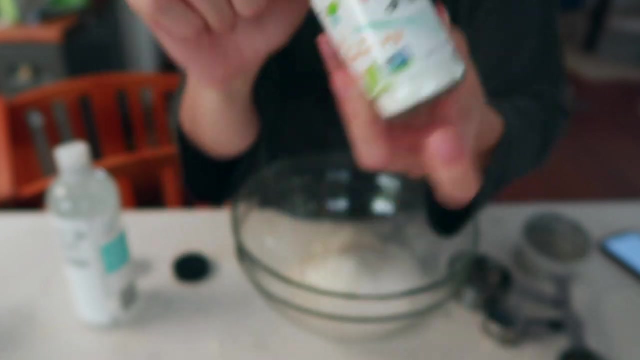 to need one cup of all-purpose flour, a quarter cup of regular old table salt, one tablespoon of oil- and you can use any oil here: Coconut oil, avocado oil, olive oil, vegetable oil- whatever you got in the pantry works. Three quarters a cup of boiling water, one tablespoon cream of tartar. 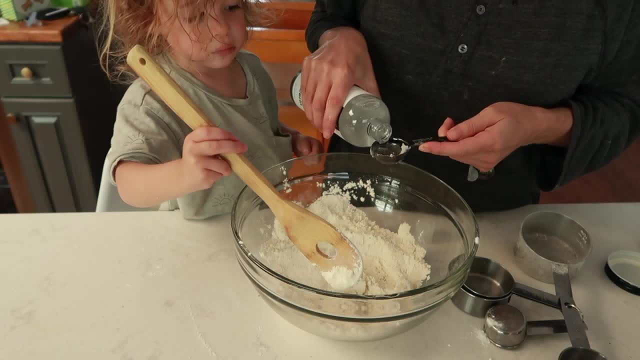 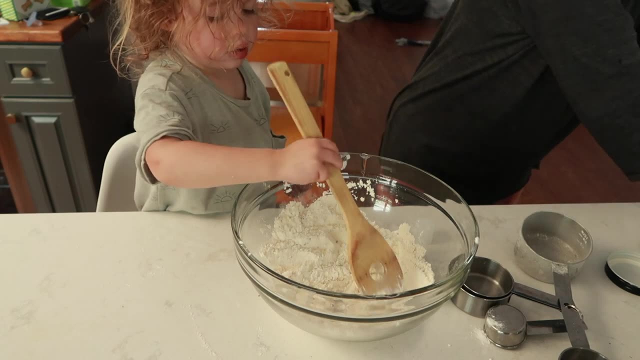 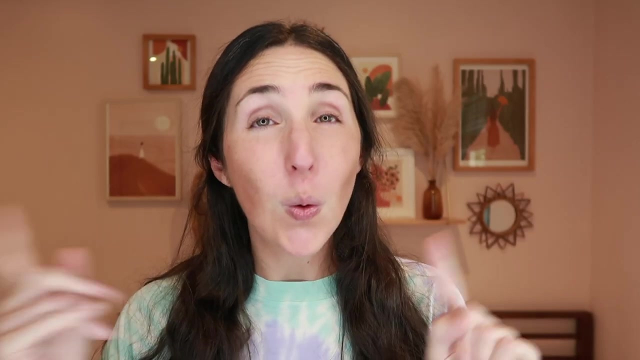 one tablespoon of vegetable glycerin- Vegetable glycerin- and you are going to use this in every meal to make your playdough. For this recipe, you are going to need one cup of all-purpose flour, a quarter cup of regular old table salt, one tablespoon of 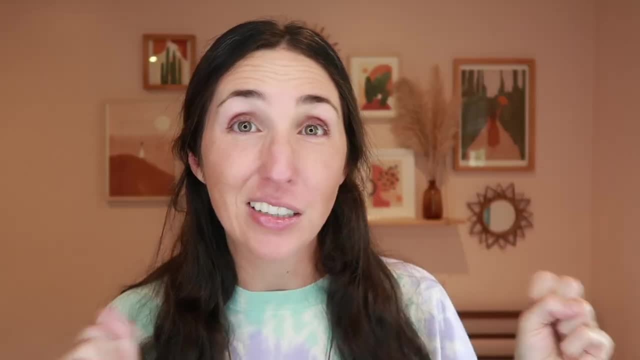 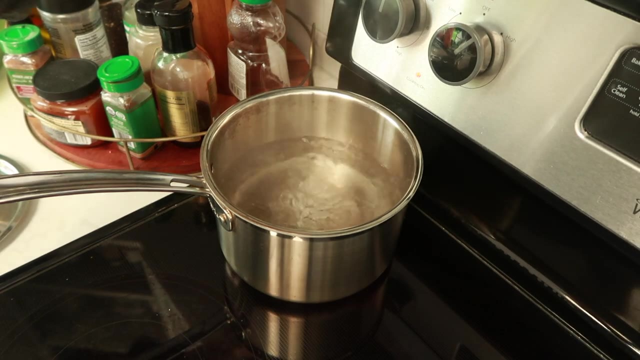 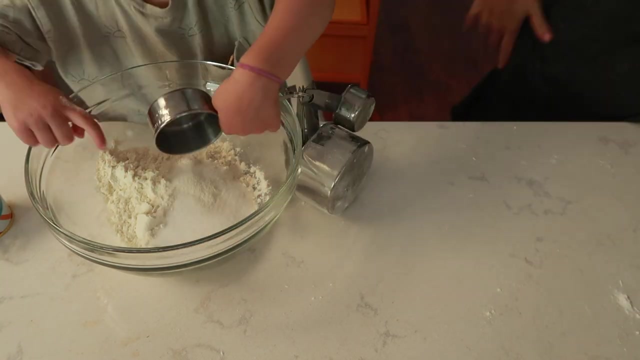 vegetable glycerin- one tablespoon of vegetable glycerin and you are going to need two tablespoons of all-purpose flour. So I am going to need one 1-in-1 ratio of all-purpose flour- one tablespoon. While you're waiting for the water to boil, in a large bowl you're going to mix flour, salt, oil, cream of tartar and vegetable glycerin. 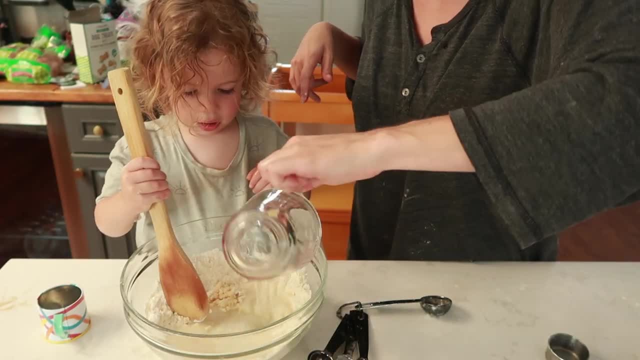 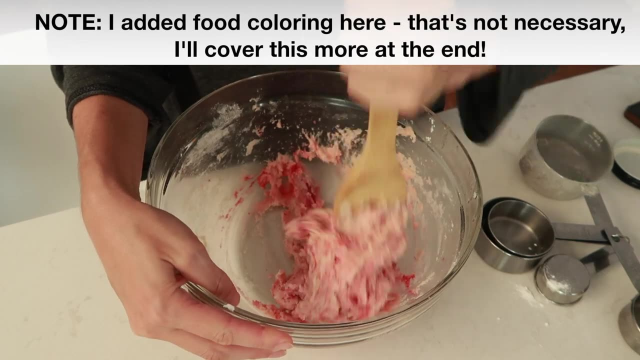 Once that water is boiling, you're going to add it to the bowl with the rest of your ingredients. You're going to mix this up pretty well and it's going to be kind of like gooey and gummy, so let it cool for about five minutes after you mix it up a little bit. 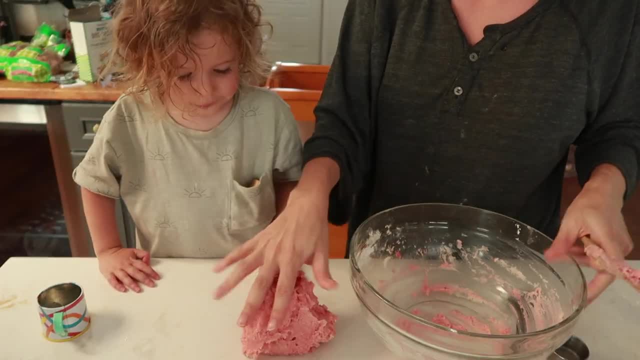 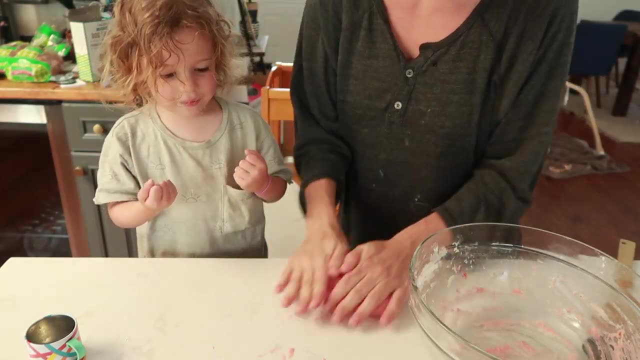 Once you can easily handle it- it's not too hot to the touch- you're going to go ahead and just knead that mixture into a nice Play-Doh ball. I have quartz countertops. They worked really well for just kneading it directly on there. 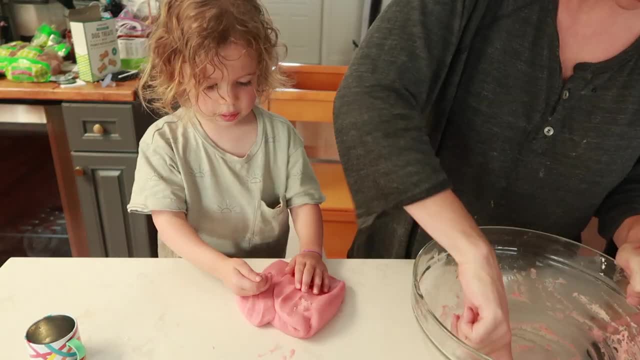 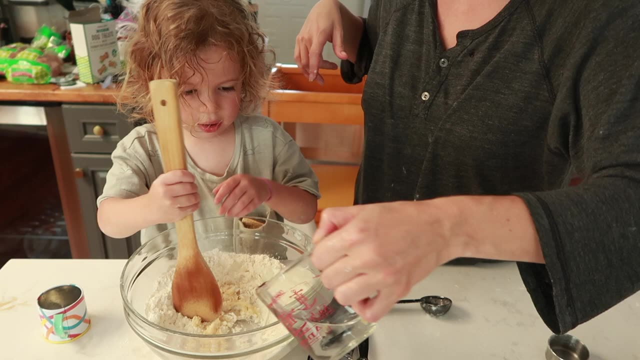 The countertop actually was cooling it. so if you have quartz or granite countertops, that should work just fine. And then, of course, you can add color. So there's a few different ways you guys can go about this. Number one: if you're making one color Play-Doh, you could add the food coloring to the water at that step. 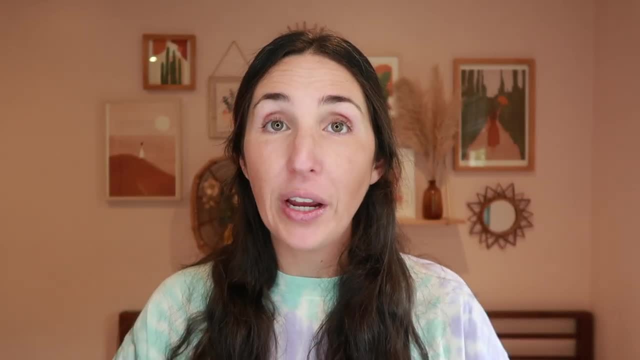 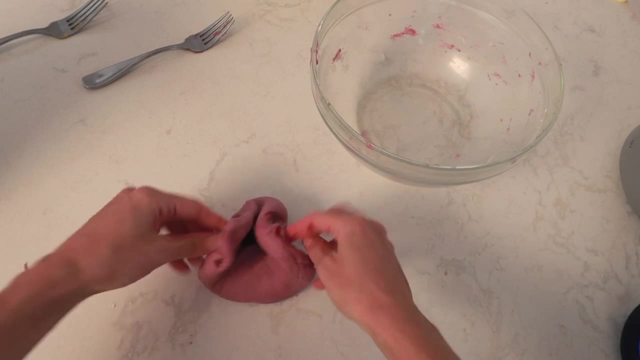 However, if you want to make multiple color Play-Dohs, you can wait and just make your Play-Doh all white and then separate and section it off and add the food coloring directly into the uncolored sectioned-off balls. 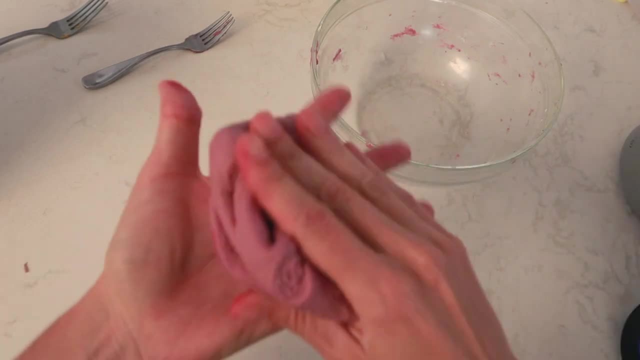 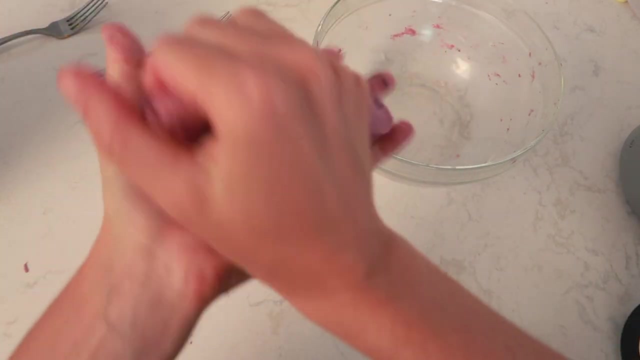 At that point you're just going to knead the food coloring into the Play-Doh ball. You could even give this to your kids to do themselves. Just be careful in case the food coloring dyes anything. but it's really simple. 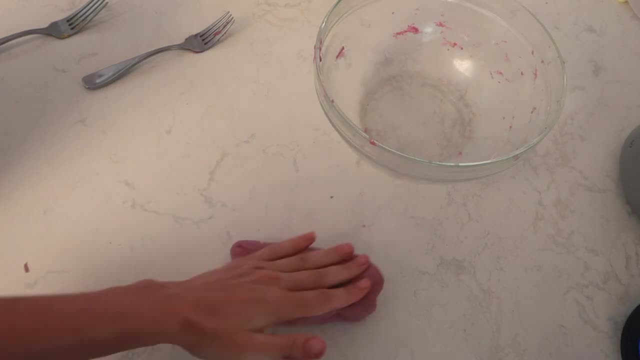 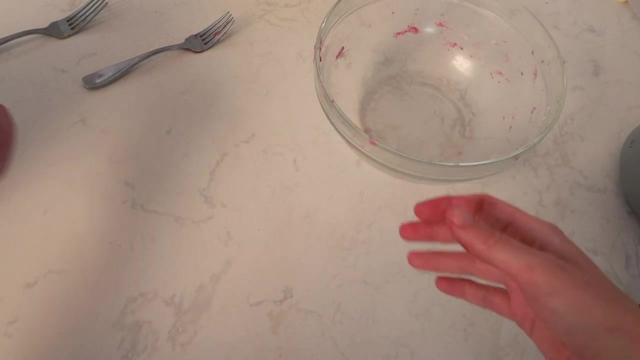 You'll just keep mixing it in until you have the desired color and consistency. I don't have exact measurements on drops with food coloring because in my experience the gel food coloring tends to be a little bit finicky. Sometimes it comes out really bad, sometimes it doesn't. 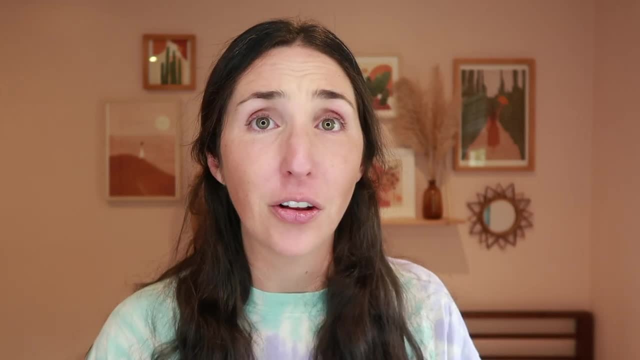 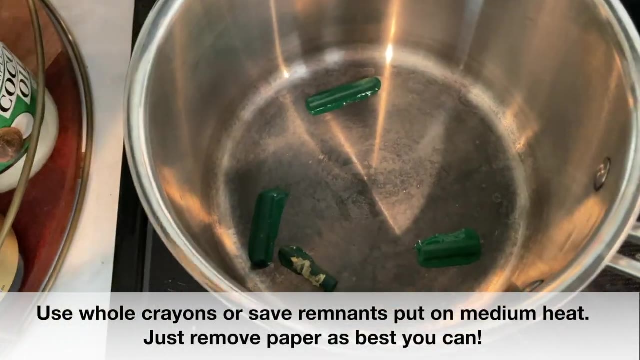 It comes out more blue. so you'll just keep adding more until you get the color you want. Or you can go with crayons. Crayons are by far going to give you the best color for your Play-Doh- the most traditional colors. 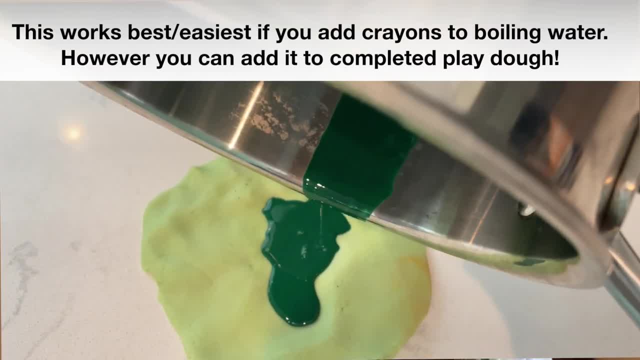 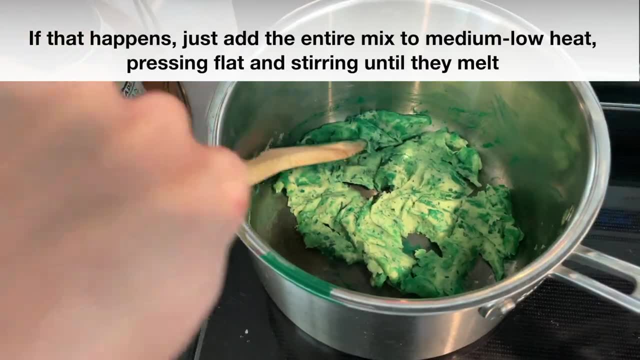 And for that you would go ahead and melt down your crayons first, and then proceed with the instructions that I already gave. And then, of course, another option would be, and you would add this in around the same time you're adding the water in. 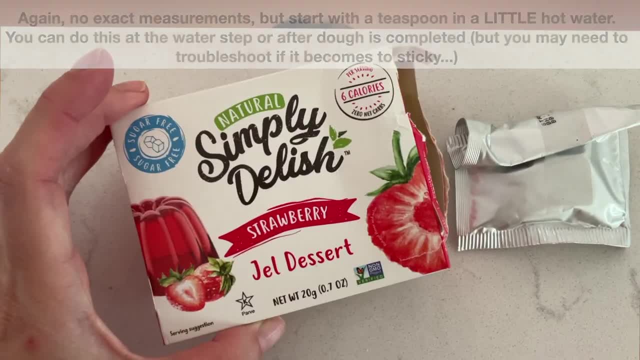 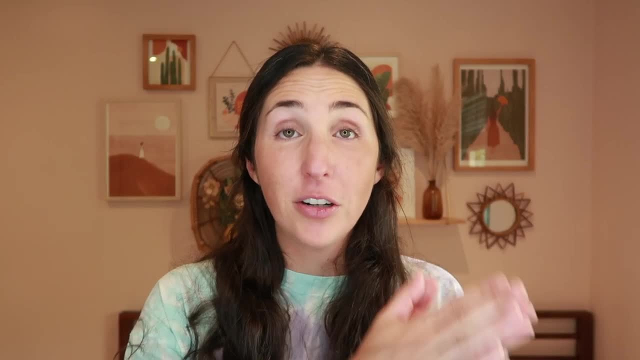 would be to just use a jello packet, a kool-aid packet, a pudding packet and, obviously, what else. Whatever color you have on hand is what color your Play-Doh will come out and be. So now, if your Play-Doh comes out too sticky, with this recipe it's super simple. 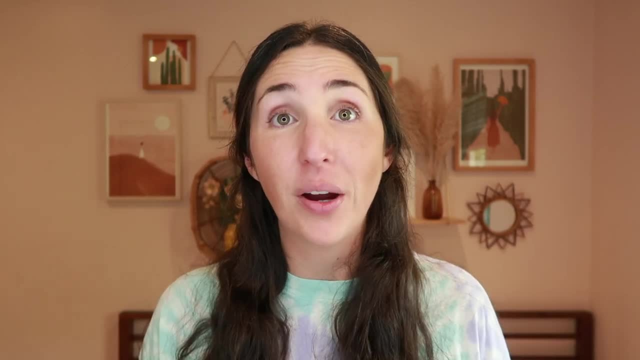 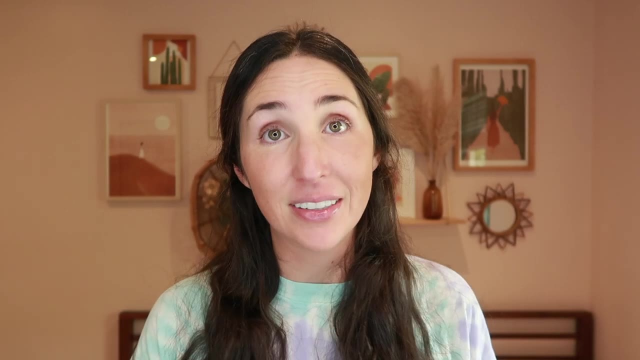 All you're going to do is add more flour. I just toss the flour right onto my counter, throw some on my hands and just re-knead it until the flour is all absorbed and you have your desired consistency, Especially if you're in a humid climate. do not be surprised if this comes out a little bit too sticky at first.